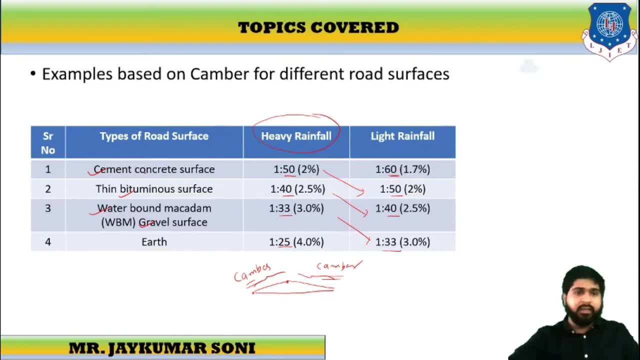 1H to 60.. If heavy rainfall is here and cement surface is there, then we need to choose this. If light is there and WBM is there, then we need to choose this road. So it is like this: This is all about camber Now. this is the example. 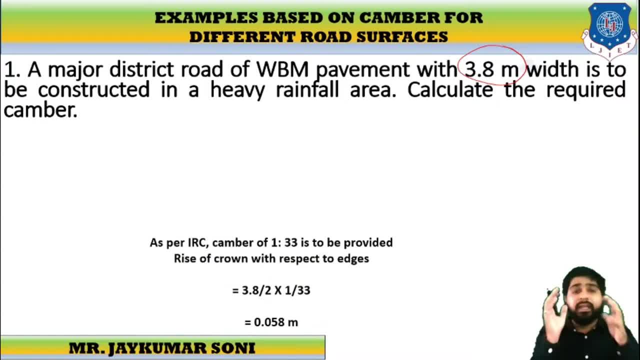 statement. What we are given over here is that a major district road of WBM pavement is there, 3.8 meter width is there, Heavy rainfall region is there. So we know that it is C, B, W E. C stands for Concrete, W stands for Water Pump, Mechanical or Gravel. 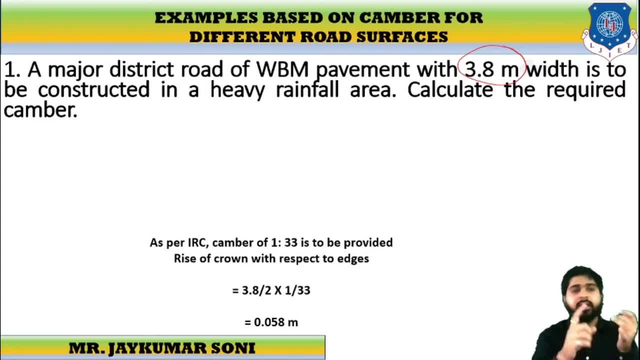 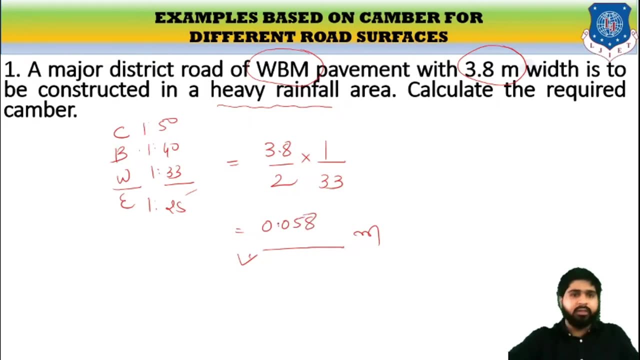 Road. B stands for Vituminous and E stands for Earthen Road. So, as per the criteria, the calculation will be like this. So this will be 0.058 meter. So this is how we can calculate the value of camber. Let us look about the another segment. another example. 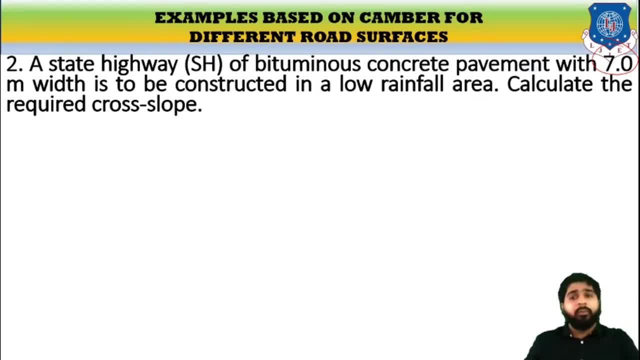 of bituminous concrete pavement is given. 7 meter road width is there. see, bituminous road is there. so it will be CBWE. out of CBWE it will be B lower rainfall. it will be 1 is to 50 and pavement width is 7 meter. so, as per IRC, 1 is to 50. we have to consider. 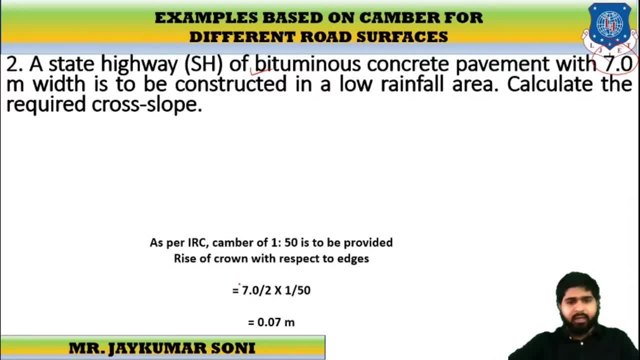 so it will be width by 2 into criteria 7 by 2, C CBWE. this is heavy rainfall. this is low rainfall: 50, 40, 30, 35, 60,, 50, 40 and 30,. it is bituminous road and low rainfall. 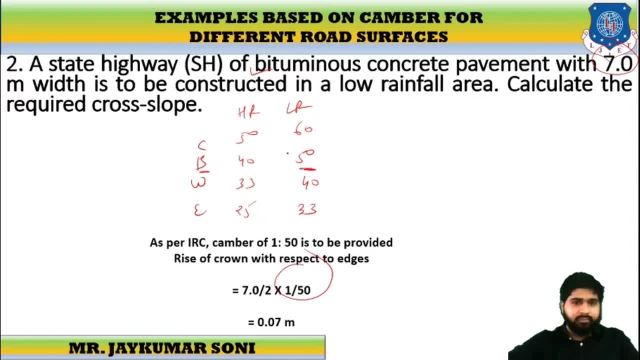 so it will be. 1 is to 50 and the pavement width is 7, which is gubernatorial, so it will be 0.07 meters. so this is how we can calculate the value of camber. I hope you have understood. 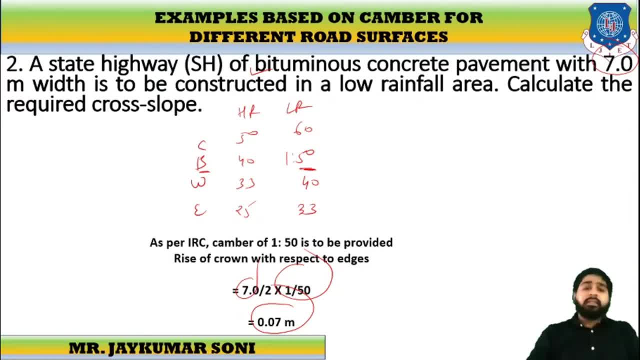 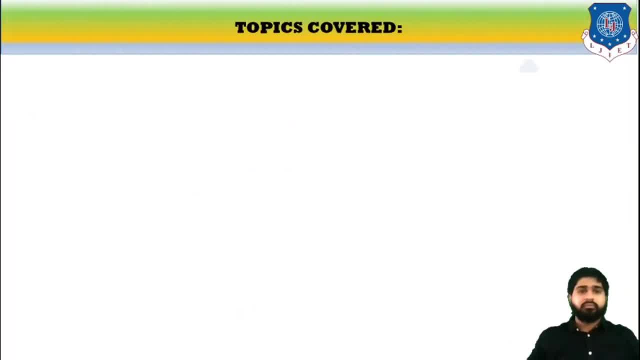 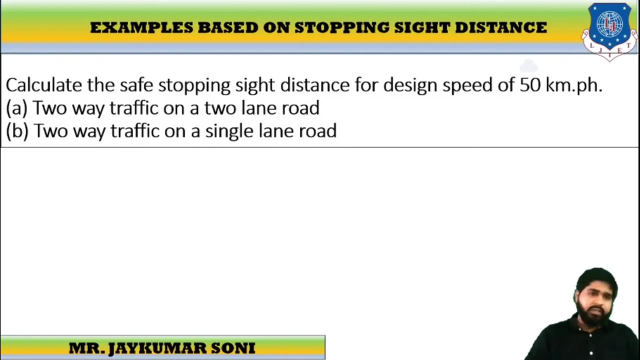 the concept thoroughly. let us discuss the another parts of this example. let us discuss about the stopping side distance. so we are going to cover the stopping side distance examples. let us understand the first statement: calculate the stopping side distance. so we have to calculate the stopping side distance for design speed of 50 kmph. first criteria: 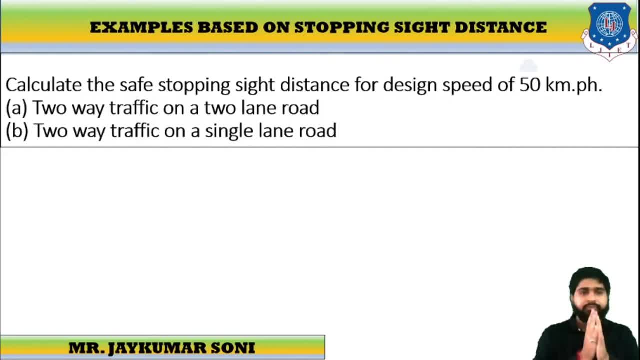 we have to calculate for two way traffic on a two lane road and another, we have to calculate SSD for two way traffic on a single lane road and we are only being given the design speed of 50 kmph. we have to calculate SSD. see, we have understood that in order to calculate, 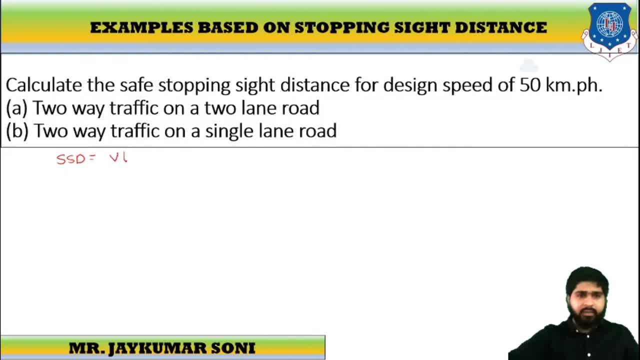 the speed we need to have. V, T, V, square 2, G, F. these are the criteria, but we are out of all these things. we are only having the design speed of kmph, 50 kmph, and we are having the speed in kmph and in our equation we made the speed in meter per second. so what? 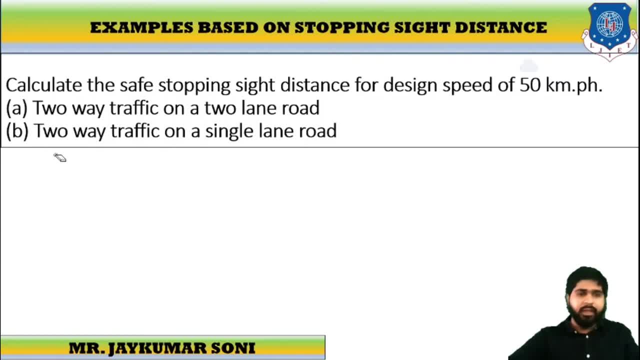 we will do. First of all, we will try to calculate the speed in kilometers per hour and in our equation we made the speed in meters per second To scribble the given values, design speed, and this is called as capital B. If I need, 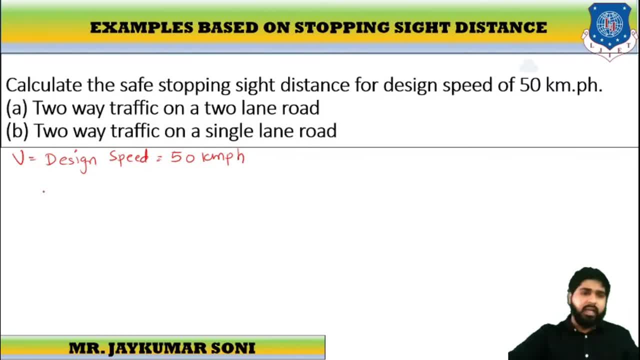 to calculate the speed in meter per second, I have to divide the kmph speed by 3.6 and I will get the value of speed into meter per second. So what is the value of meter per second? It will be 13.9 meter per second. This is the first thing Now we need to have. 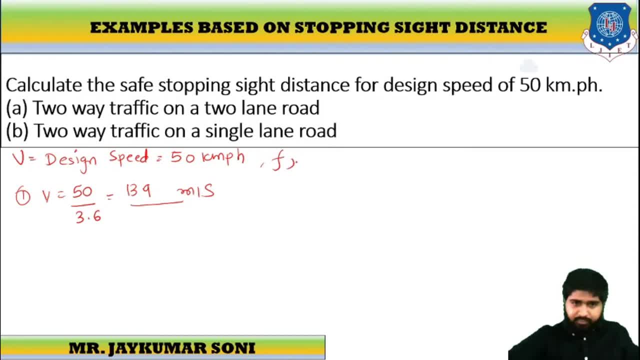 the assumption of F, the value of G and the value of T. I have already described that if we do not have the value of T, then we can consider it, So we will take it as 2.5 seconds. So this is the. we have the value of G as 9.8 meter. 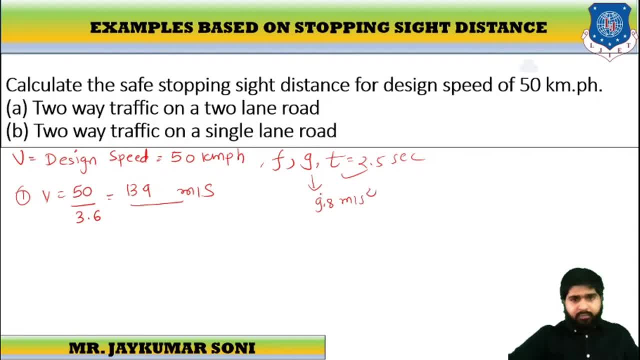 per second square. We have the value F from the range of 0.35 to 0.14, we will take it as 0.3.. So let us put it first. The first is about two-way traffic on a two-lane road. 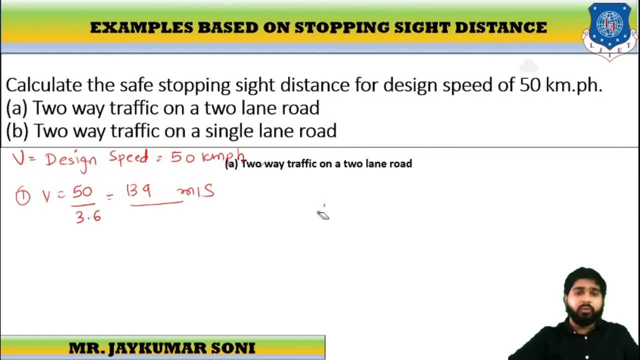 If it is two-way traffic on a two-lane road, then the example calculation is very simple. It is: SHD equals to VT plus V square by 2GF. V- we have calculated over here- is 13.9.. T. 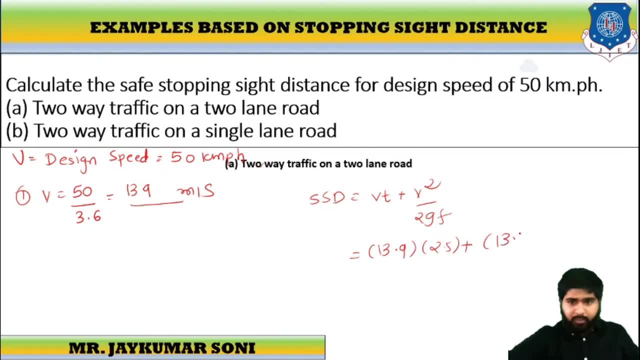 is 2.5 plus it is 13.9. whole square by 2 into 9.81, into F stands for 0.. Let us calculate this value, What you are getting. just calculate It will be 61.39 meters. So this is when we are discussing about two-way traffic on a two-lane road. 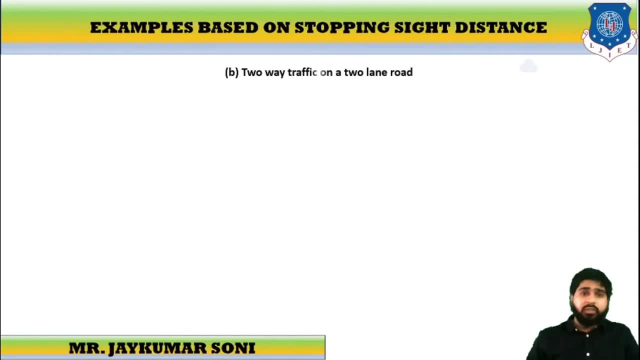 But if we are talking about two-way traffic on a single-lane road- this is single-lane road- Then it will SHD will be twice of the calculated SHD, So it will be twice of 61.39.. So it will be 122.39 meters, 39 to the 78.. So this is how we can calculate. 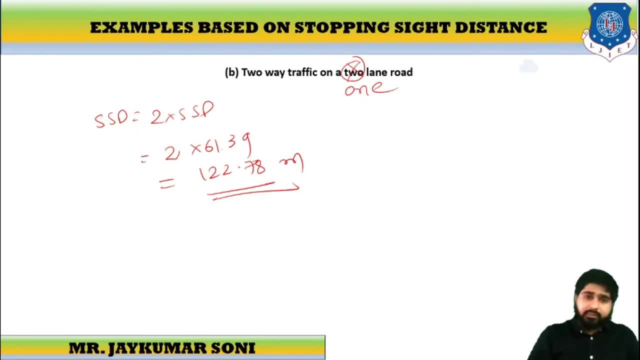 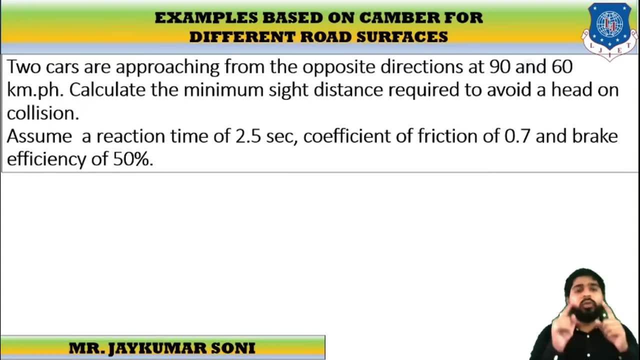 the values of SHD. Let us move towards another example. Okay, another method. This is the statement: Two cars are approaching from the opposite direction. One is at 90 kmph and another is at 60 kmph. So we are having two values of V, V1 and V2.. 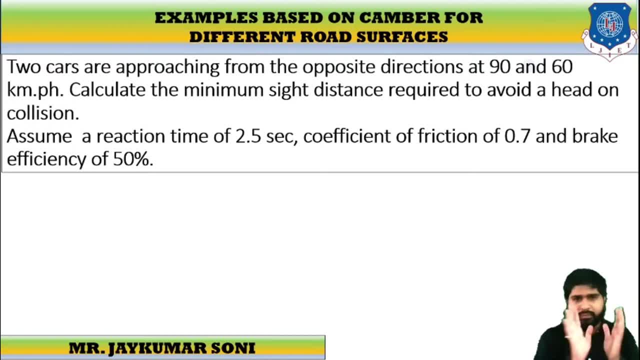 So we need to convert both of these values in meter per second. This is the first thing. Then we have to calculate the minimum SSD to avoid the hedon collation. We are given the value of T, that is, 2.5 seconds. We are given T is equal to 2.5 seconds, F is equal. 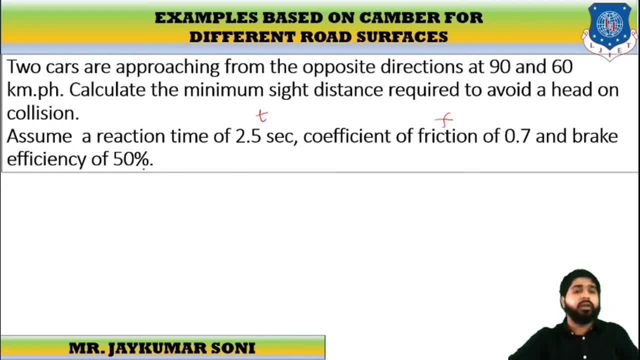 to 0.37 and brake efficiency is 0.5.. See, first of all, we are given the value of V1 as 90 kmph and V2 equals to 60 kmph. What we will do: Divide it by 3.6.. Calculate and tell me what are the answers for this. Okay, so this is. 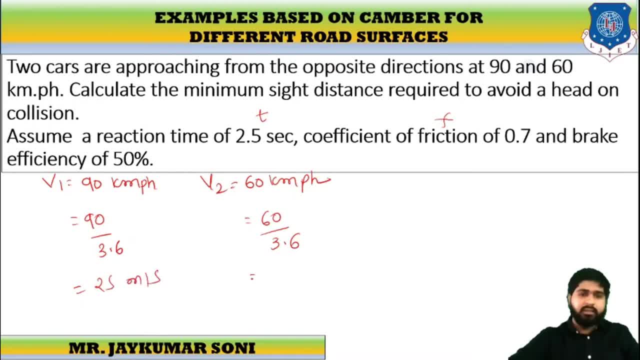 25 meter per second and this is 16.67 meter per second. V1 and V2, we have calculated, Fine. Now we have to calculate the value of SSD. So we are having two values of V- V1.. So we will calculate two SSD: SSD1 and SSD2.. But one thing that we need to understand over: 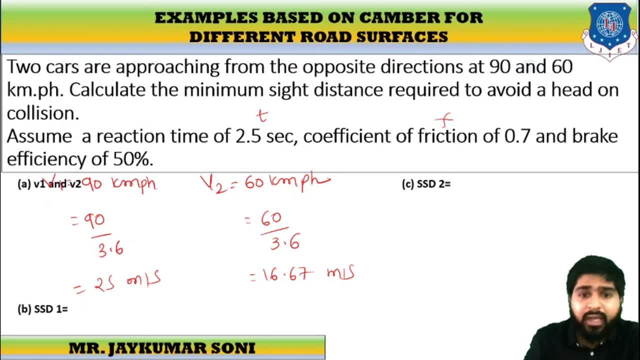 here is. we are given over here. let us conclude this. this small v1 and small v2, so that it cannot consume more space on the slide, See small v1. we have calculated as 25 meter per second and small v2 as 16.67 meter per second. 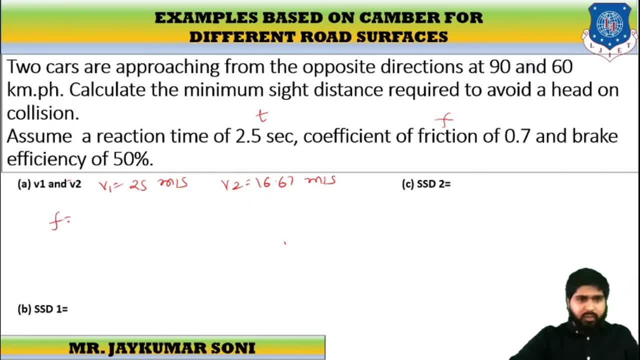 Now we are given over here F. the value of S is 0.7.. But here the statement is written over here that brake efficiency is 0.50.. So only half of this efficiency is working. So it will be 0.35.. We have given the value of T as 2.5 seconds. What we will do, We will. 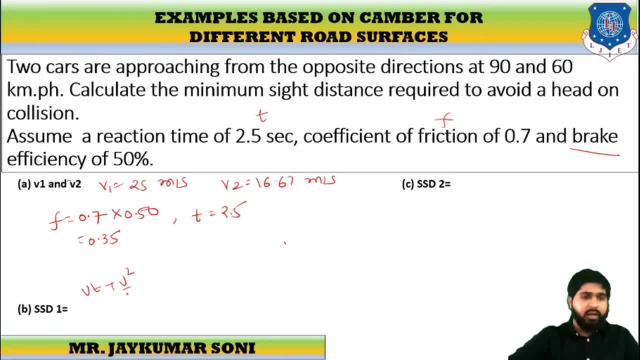 calculate SSD1.. That will be VT plus V square by 2G. error: That will be 25 for V1, 2.5 plus 25 whole square by 2, 9.81 into 0.35.. For V2 it will be 16.67, V into T, then 16.67 whole. 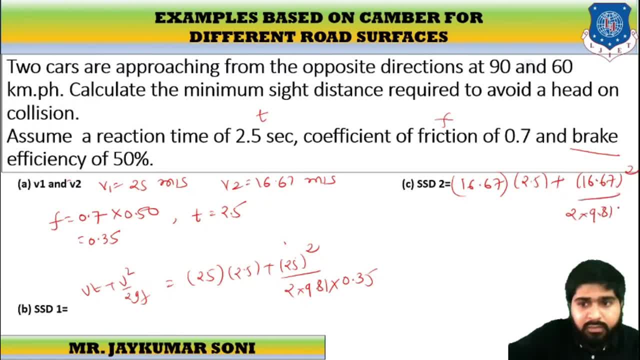 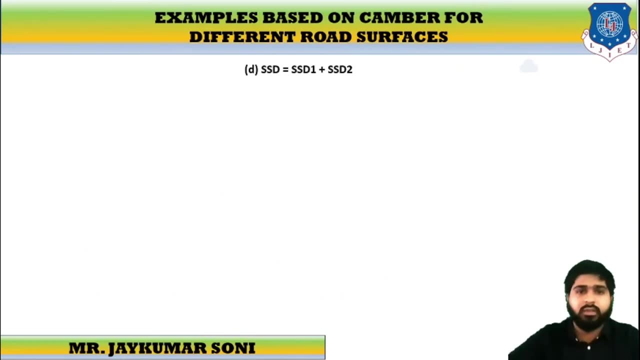 square by 2G into Calculate this value and tell me what is the ultimate answer. So we are given over here F. Tell me what is the answer. SSD1 is and it is, so it will be 0.20,. this will be 5.. This is the total SSD that we are getting over here. So we have understood. 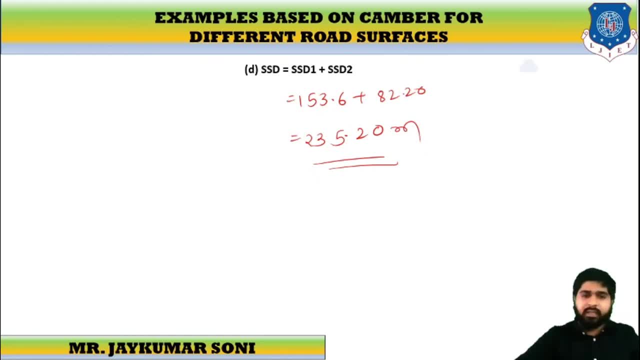 the construction. Thank you. Conceptually, what we have done in this example, we have converted a V1 that was 90 by 3.6.. So we have converted that, Then we have converted a V2.. Then we have considered F with the brake. 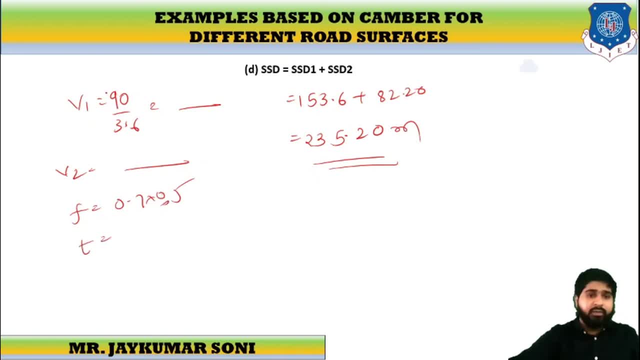 efficiency. We have been given the value of T, We have considered SSD1 for this V1 and SSD2 for this V2.. And then we have added these two values and, final, the ultimate SSD value is 235.. Let us move ahead with another example. See, this is the example statement. So this is: 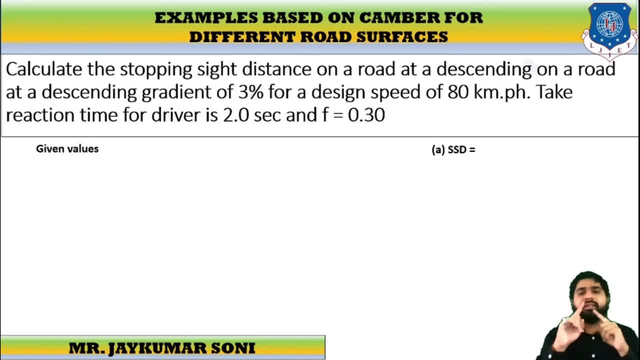 the another example statement: Calculate the stopping site distance on a road at descending gradient. Descending gradient is given over here. So it is like this: the road is like this: in this direction, 3% descending gradient is given. the value of N stands for the road. 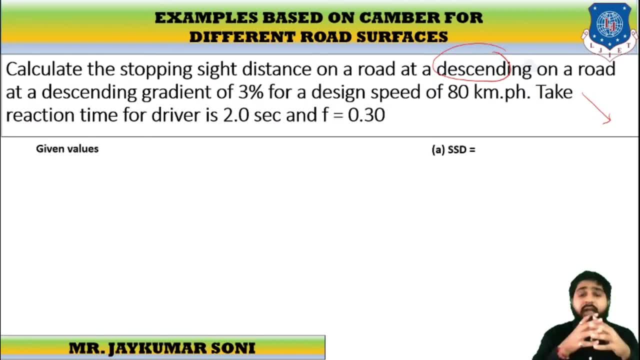 So this is the number so far. Now let me calculate the distance. heaven, You will see, it is given over here. So this is the number of roads and that is given over here. Now the value of n stands for 3.. Design speed is 80 kmph. Take reaction time. t is equal. 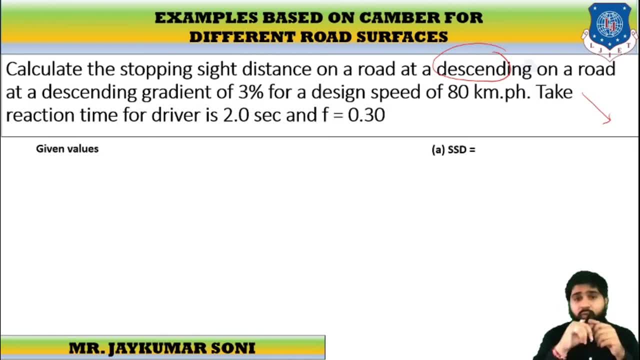 to 2 seconds Instead of 2.5, it is t, t is equal to 2 and f is equal to 0.3.. So what we are given over here is we have been given value. of v is equal to 80 divided by 3.6, and